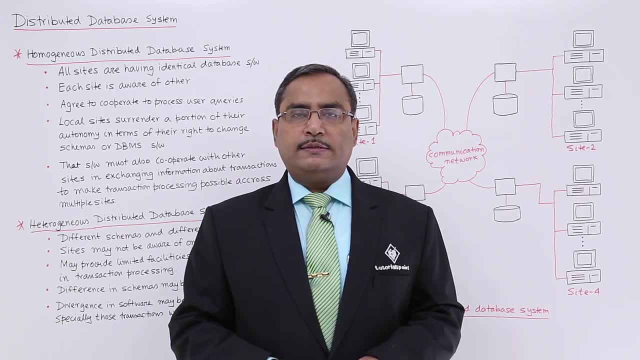 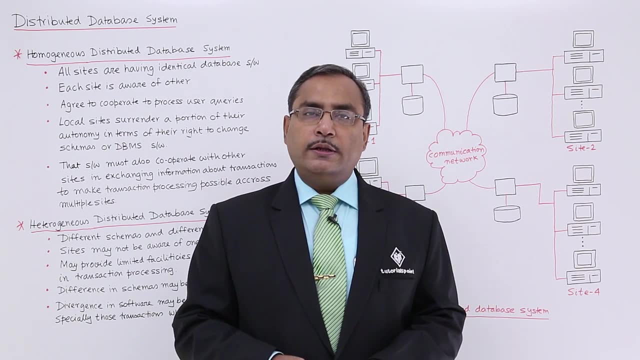 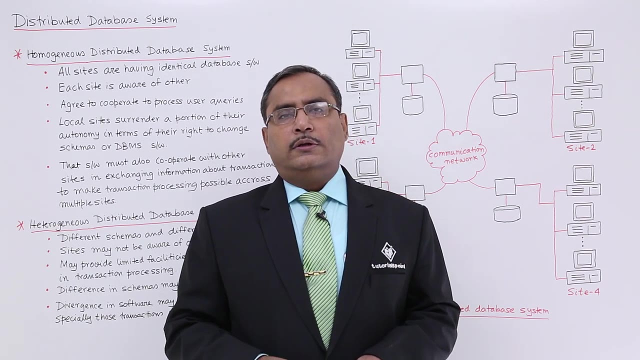 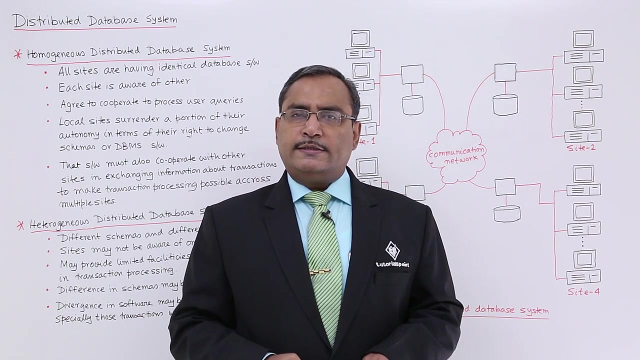 We are discussing the topic distributed database system. In the earlier video we have discussed what is the distributed database system, what is client server model, decentralized model and centralized model. So here in this session we are concentrating only on distributed database system. We know that in case of distributed database, logically connected single database. 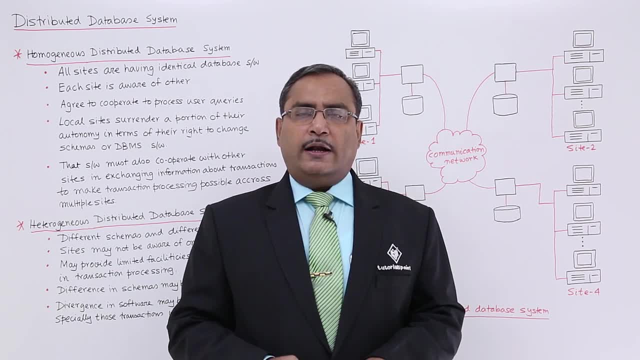 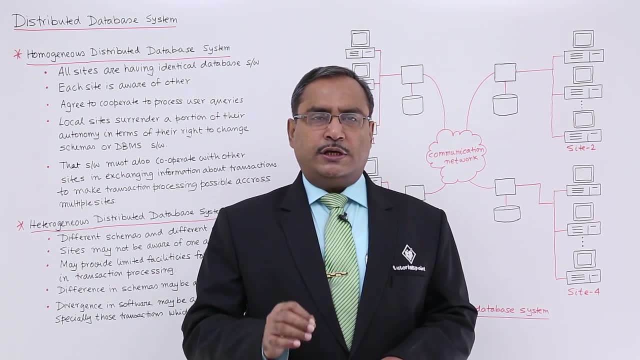 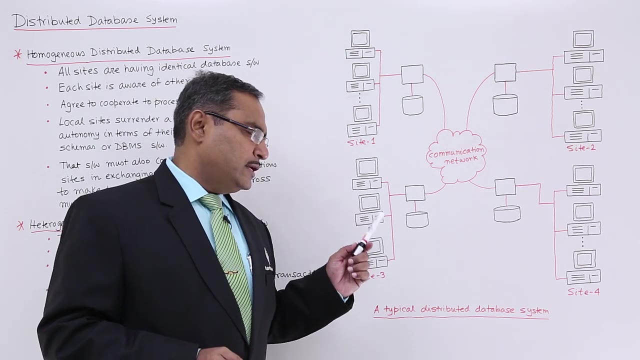 dispersed at different sites and all those sites are connected by computer communication network. So that was the basic definition of distributed database. If you can look at this particular diagram, you can find we are having site 1, site 2, site 3 and site 4.. 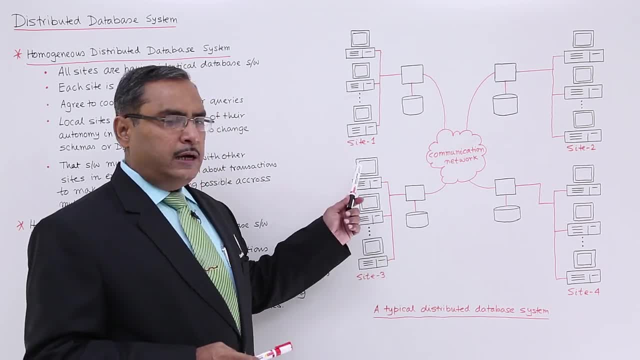 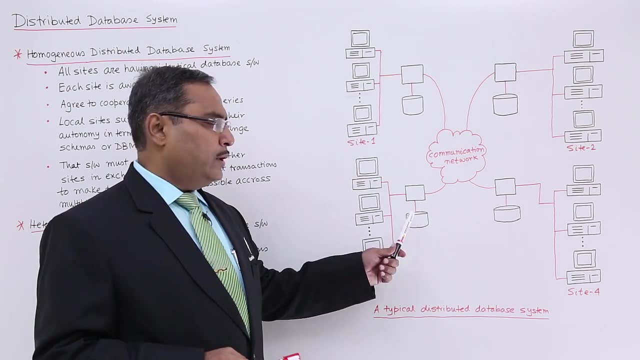 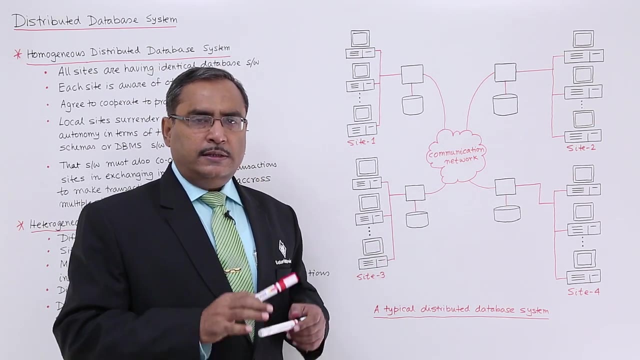 Four sites are there. Each and every sites are having multiple client machines and there is one server is there And this server is having the respective disk storage where the database is, And all these sites are having the distributed database. That means the database has got. 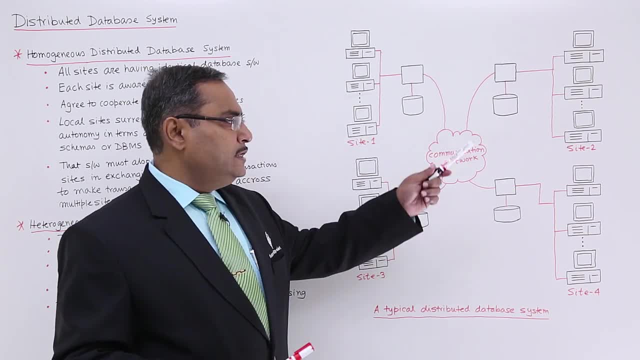 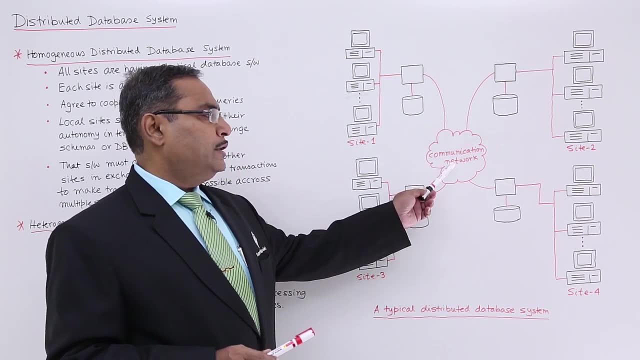 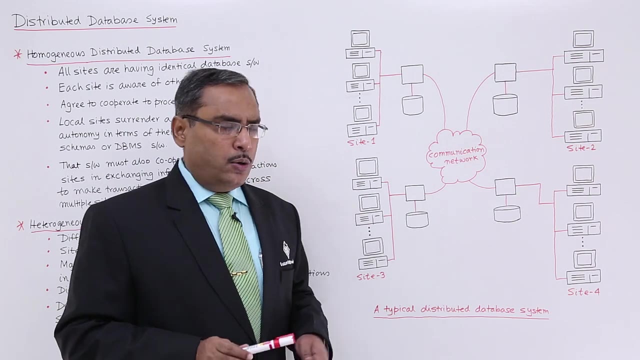 divided and distributed and dispersed in these four sites. All these sites are connected through computer communication network, So that is the communication network with the help of which all these sites are connected. So in case of distributed database, whenever one query will be produced from one of the users, then the query will be distributed. 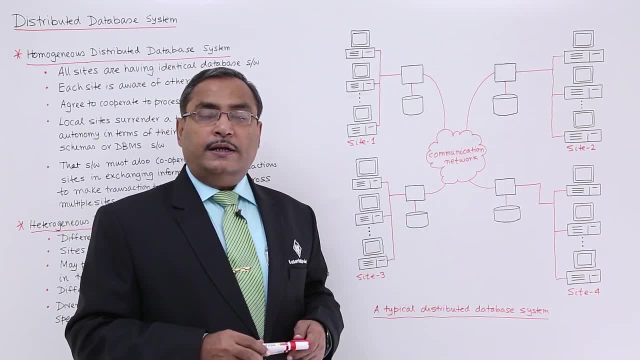 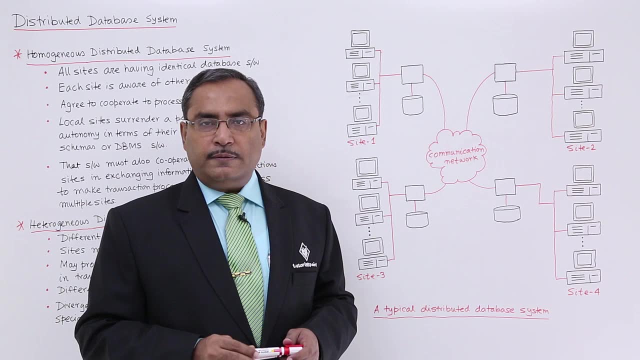 to the other user. So in case of distributed database, the query will be processed from the local database If the respective portion of the database required for the processing of the query is available at the local server. If the corresponding database is not available, 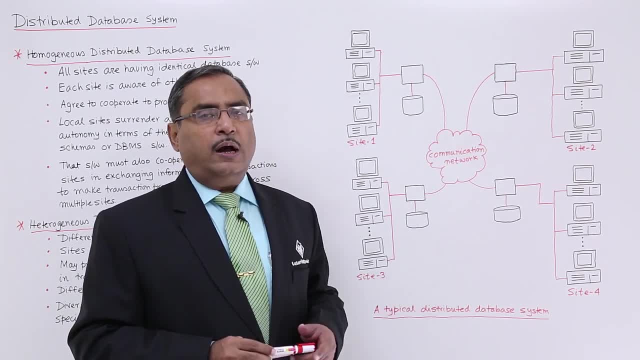 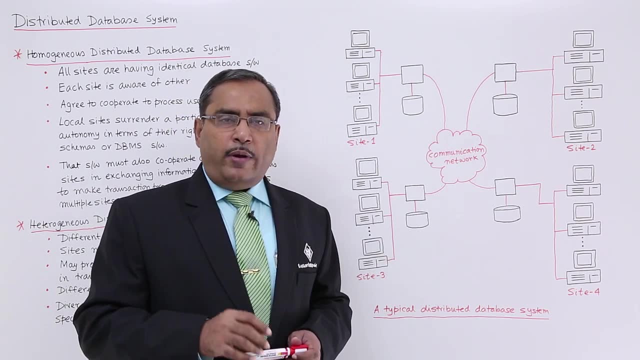 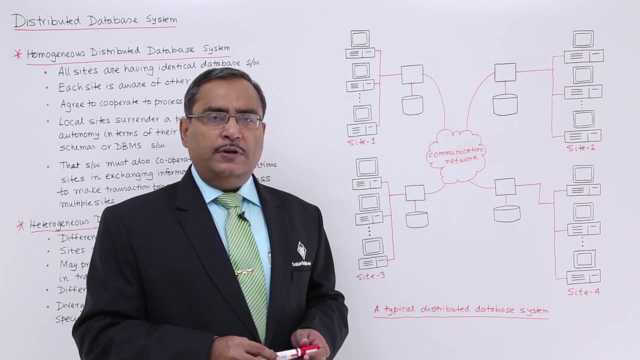 then the database will be accessed from the distant servers through this computer communication network, But from the client end it will remain transparent. Each and every query execution in distributed database will be- seems to be- local. So in case of distributed database the client will feel that whatever the query has got processed and generated by himself. 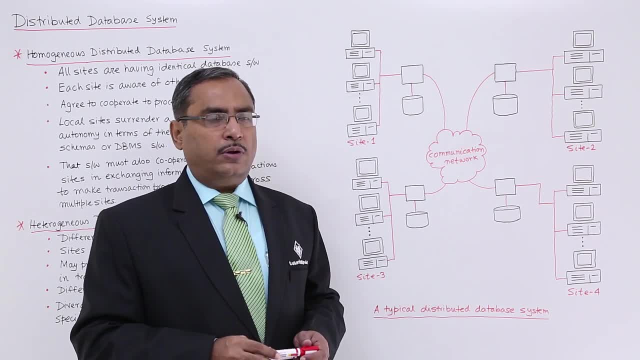 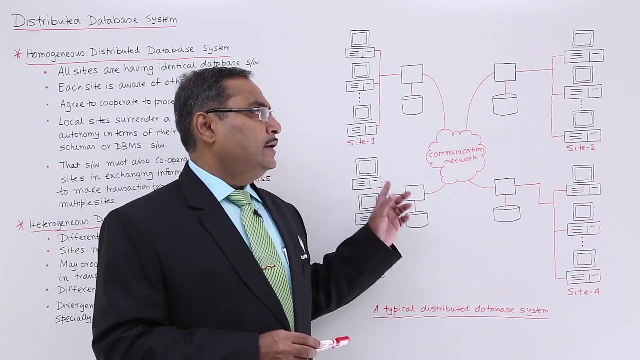 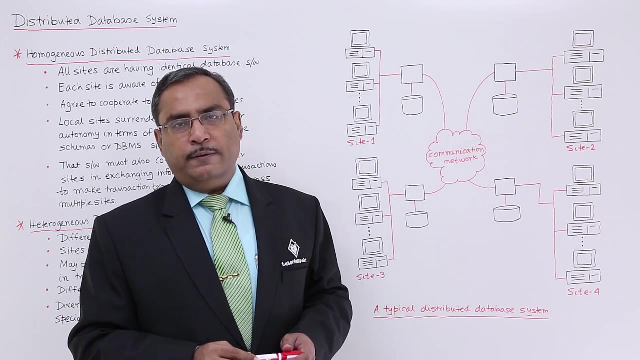 or herself was done by the local database only, And that is also a very important issue. And in case of distributed database, all these sites, the respective databases, will have their local rights, will have their local rights, And that is also important as one. 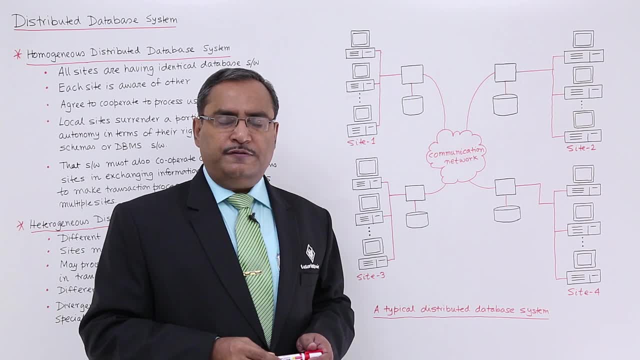 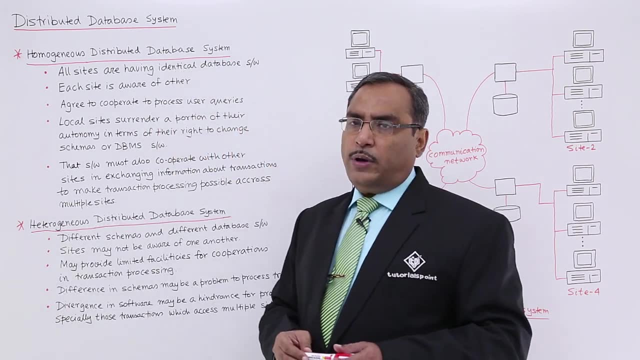 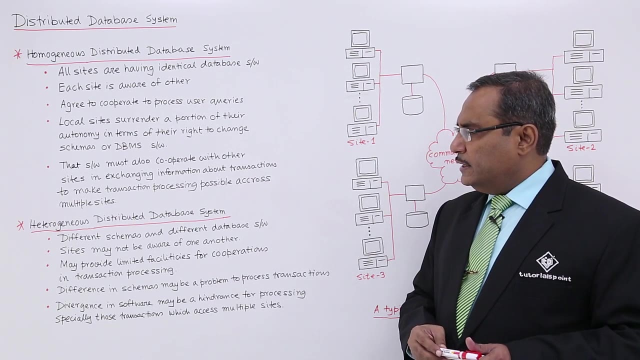 of the features. In the next video also, we will be discussing different other features and advantages of distributed database. This distributed database can be mainly divided into two categories. One is your homogeneous distributed database system And another one will be the heterogeneous distributed database. 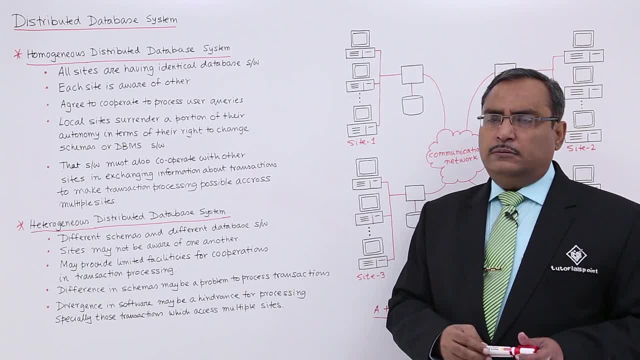 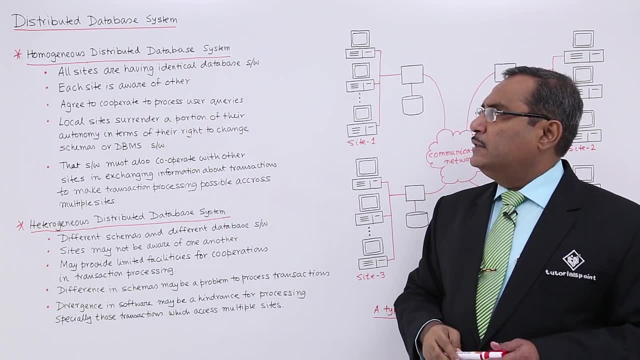 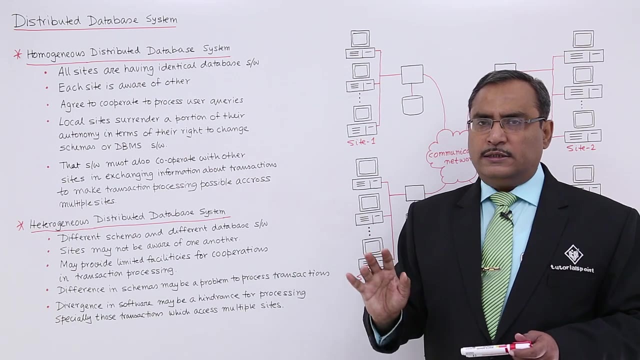 system. Okay, Now let me cover the homogeneous part at first. So homogeneous distributed database system. All sites are having the identical database software. So whatever the database softwares are there installed, All the sites are having the same database software. That is very important, Each site. 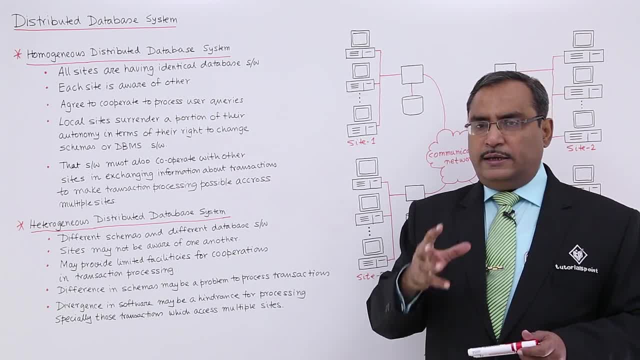 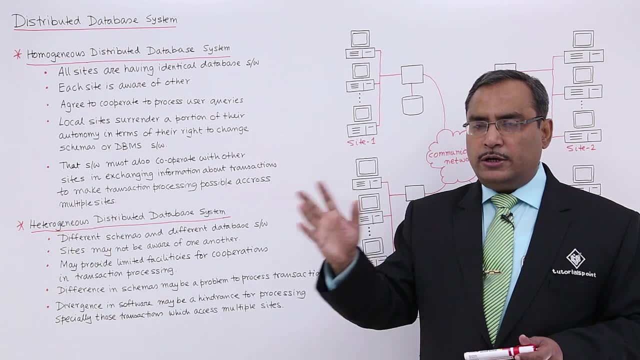 is aware of other. Each and every site knows that they are having the partial database. Other database is having two other sites And they know what are the other sites. are there containing the part of the databases? Agree to cooperate to process user queries. 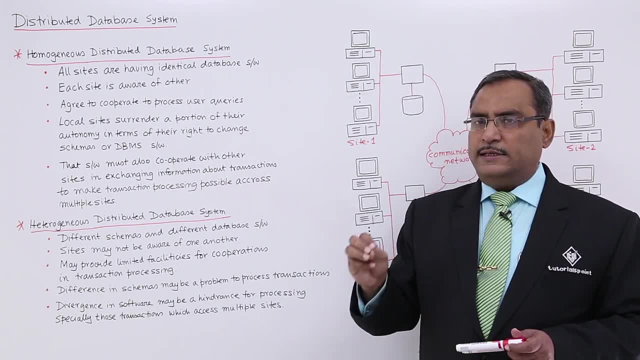 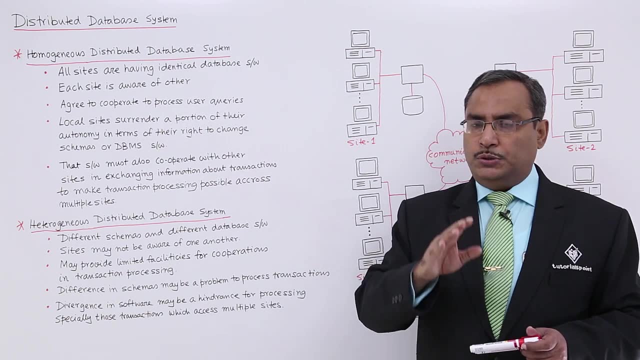 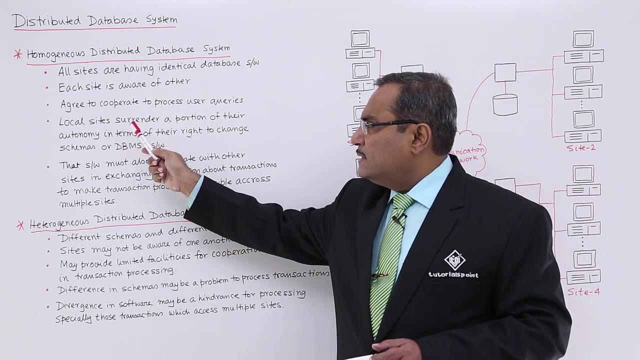 Whenever a particular query will come which is required to have an access over the different databases On different sites, and these sites will be in a mood to do the cooperation. So agree to cooperate to process user queries. Local sites surrender a portion of their autonomy. 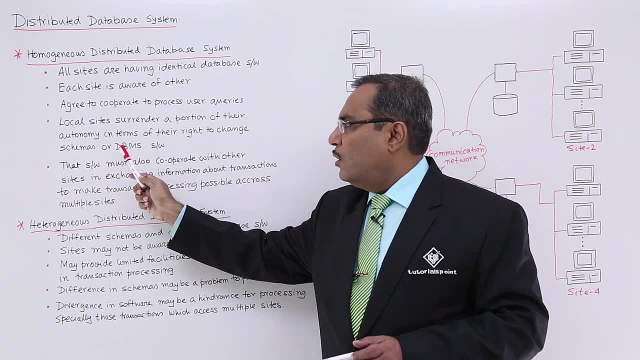 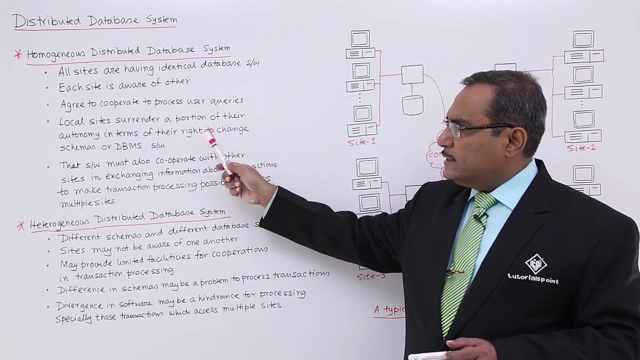 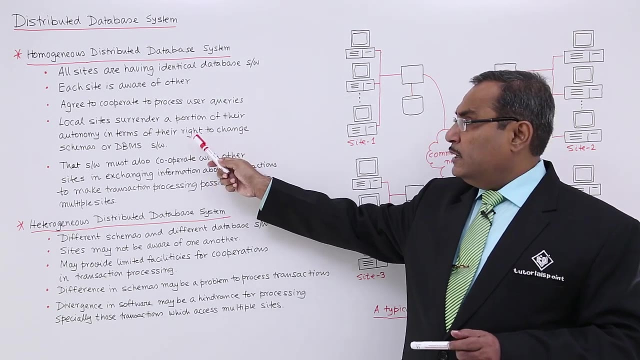 in terms of their right to change schemas or distributed database management system softwares. So I told you that, in case of distributed database, each site is in its own right. So in its own right, Good. But so they are surrendering a portion of their autonomy in terms of their right. 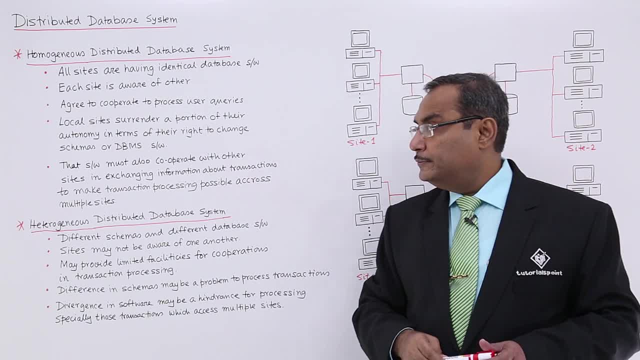 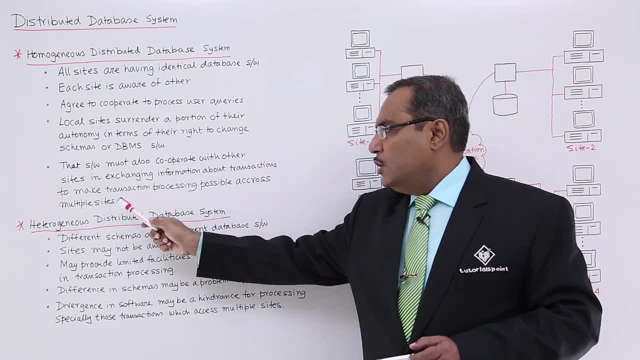 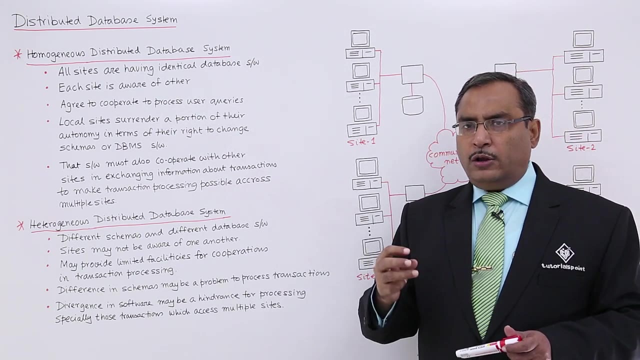 to change the schemas or DBMS software. The site must also cooperate with other sites in exchanging information about transactions to make transactions processing possible across the multiple sites. I told you this one earlier also that a particular query may be accessing different tables, different schemas, different relations. So the process in which the different databases are being 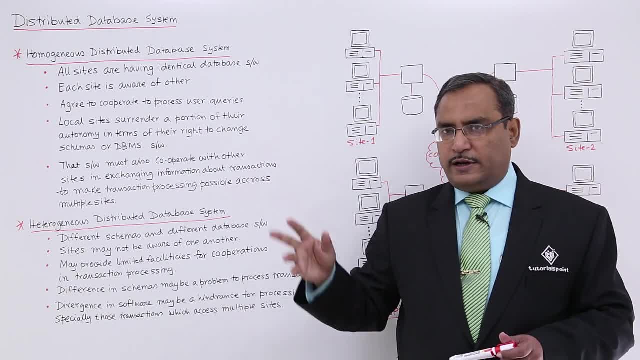 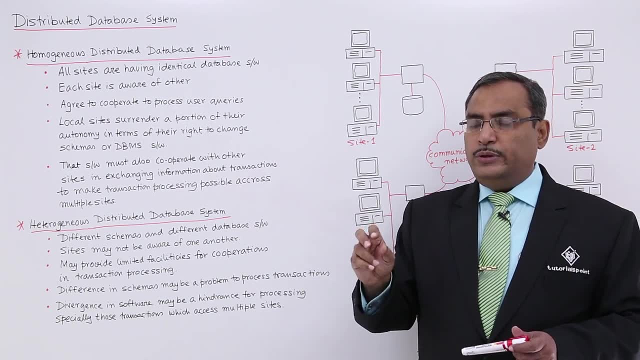 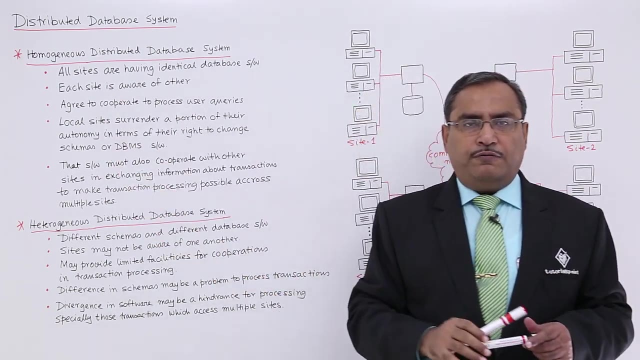 And those relations or tables are distributed onto different sites. So these particular sites are in a mood to agree with the cooperation to be done for the processing of those queries. So this is our main features of homogeneous, distributed database system. Now let us go for the heterogeneous one.